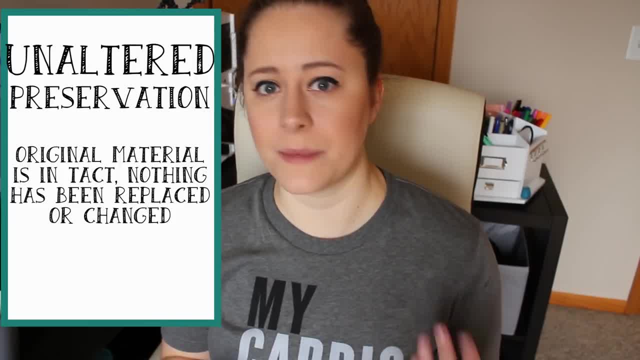 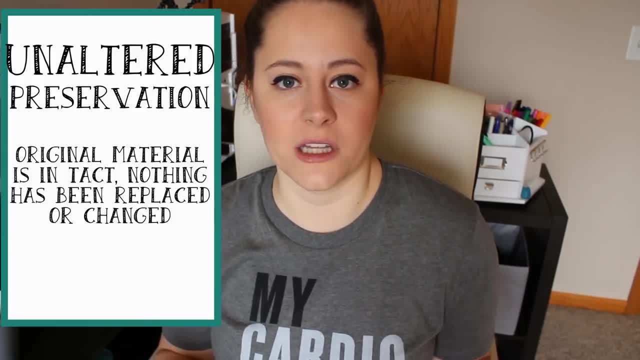 where something doesn't change at all. This happens when we get bugs trapped in amber, but another famous incident is from the La Brea Tar Pits, where we had saber-toothed cats that basically were completely unaltered when we found them. Next we have permineral. 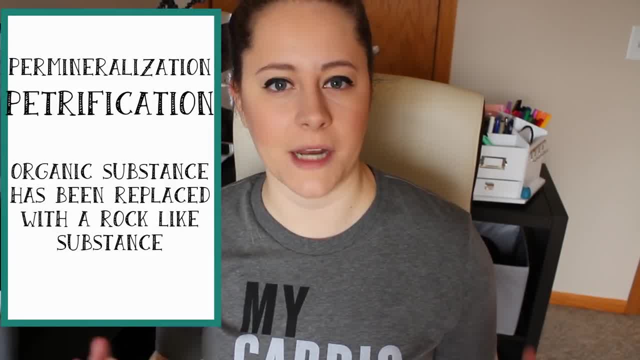 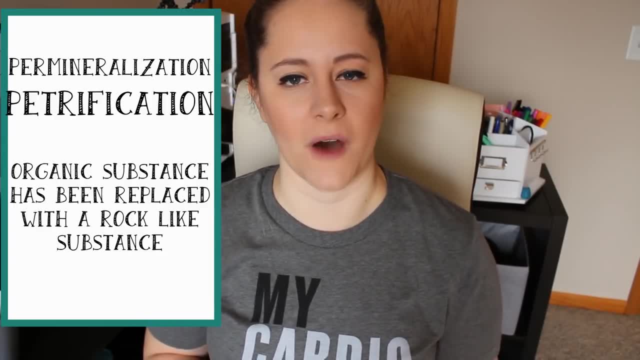 permineralization or petrification. What that means is that whatever made up the organism has been replaced by a mineral. Petrified wood is a really good example of this, as are most bone fossils. Permineralization or petrification can happen to both hard and soft material. 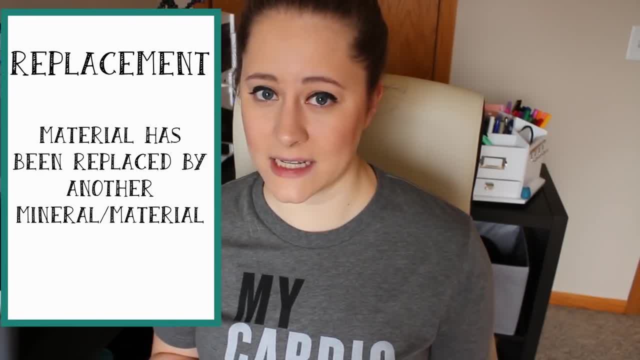 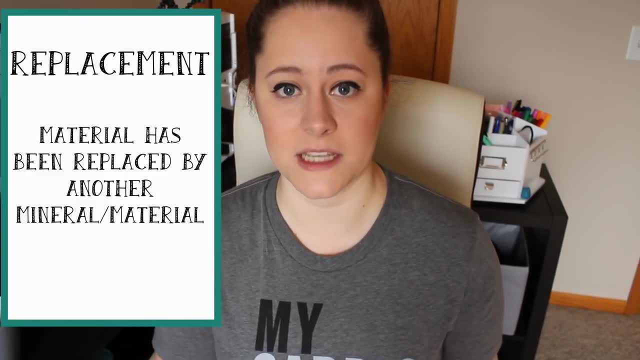 Replacement is another method in which something will become a fossil, As the name suggests. this is where one mineral is replaced by another. It's important to note that if a material disintegrates first and is then replaced, we then have a cast fossil. Next we have carbonization. 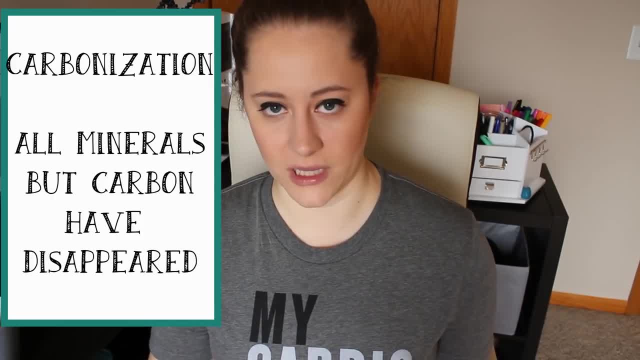 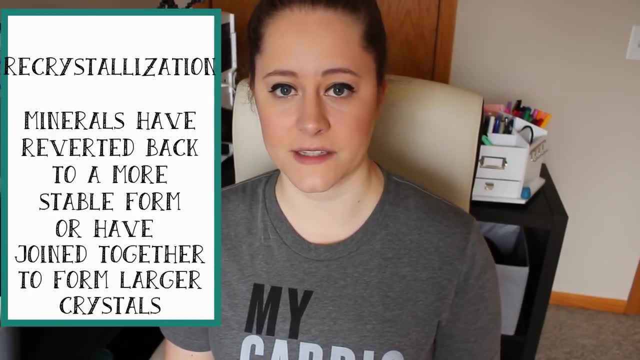 This is when everything else has been removed except for carbon and you're left with just a hunk of carbon, which is what coal is. And finally we have recrystallization. This is a fossil where minerals have reverted back to a more stable form or have joined together. 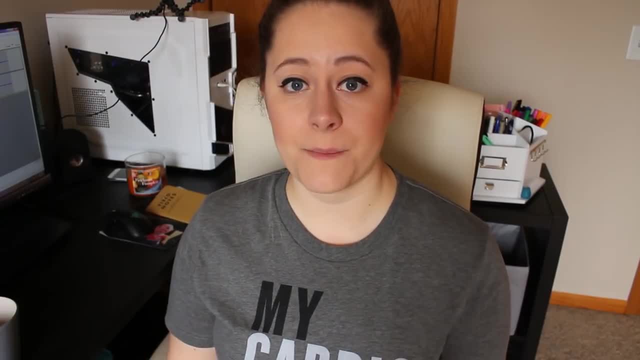 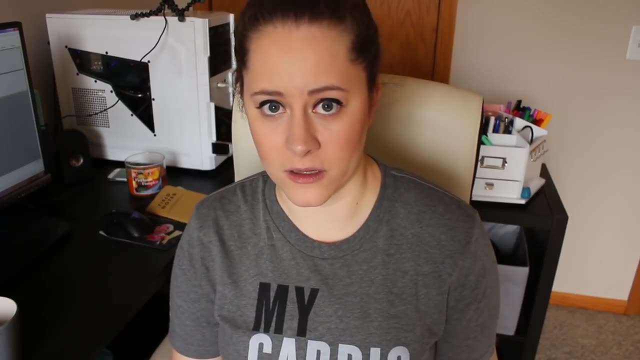 with other crystals to form even larger crystals At the base of fossilization. there is a list of things that need to happen. A part of an animal or a plant or an object falls. It is then covered up very quickly. If it is not covered up, then a lot of what could be. 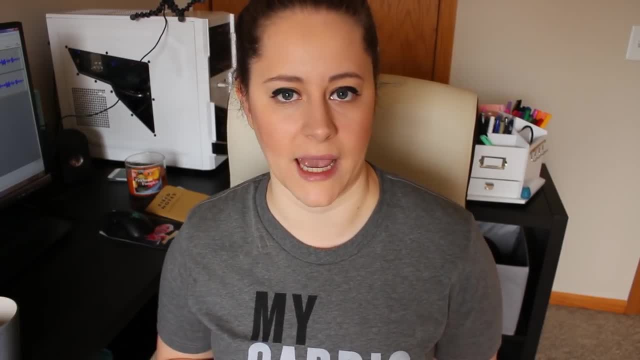 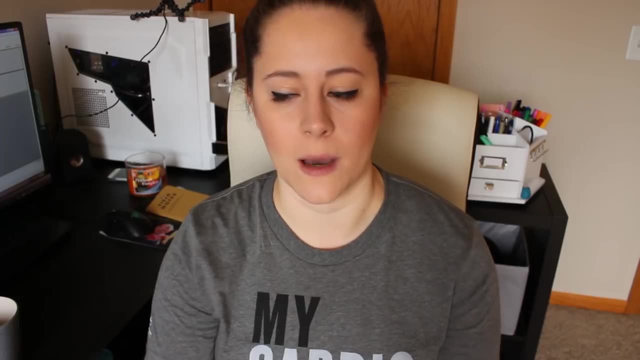 preserved will be lost either due to animal activity or just simple decay. So next time you're standing in front of a fossil, think about all of the different things that needed to line up to get it to that museum or to that display or to that side of the road where you found it. Think. 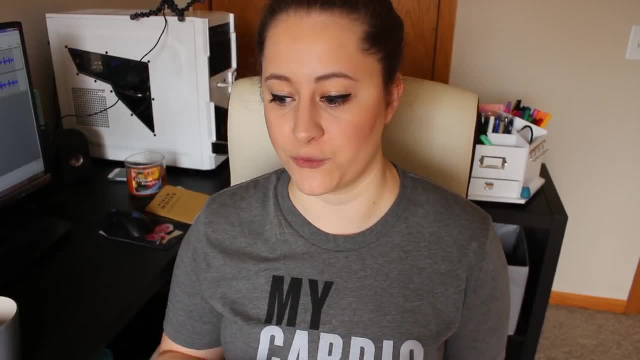 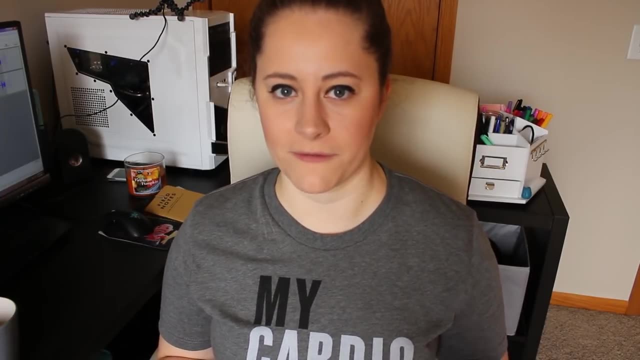 about what kind of fossil it is. Is it a cast of something? Is it a bug preserved in amber? What kind of fossil is it? I hope this has been helpful in determining what kind of fossils are what. What have been some of your favorite fossils? I've made a video about two of my favorite fossilized things. 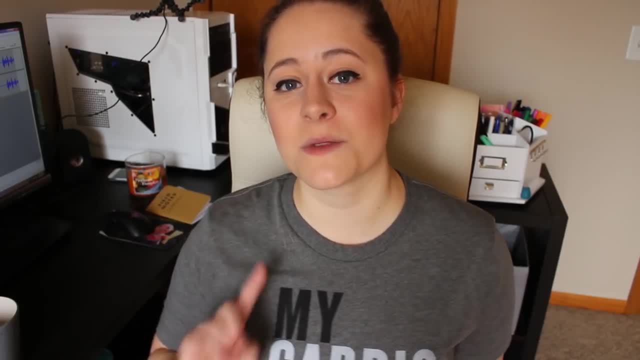 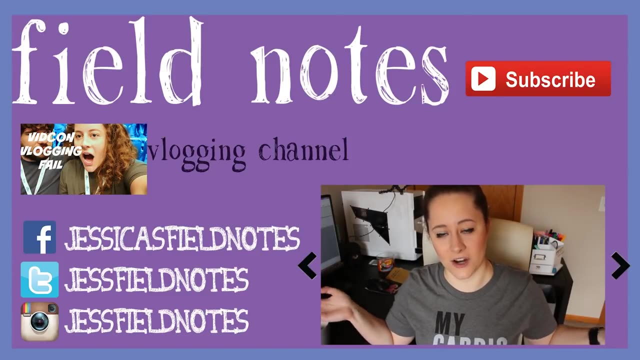 Remember to hit like if you like this video, subscribe if you would like to see more, and I will see you guys next time. By the way, I wanted to talk about this here in in the end card, in case you've stuck around. I've seen that there is a very high percentage of my external